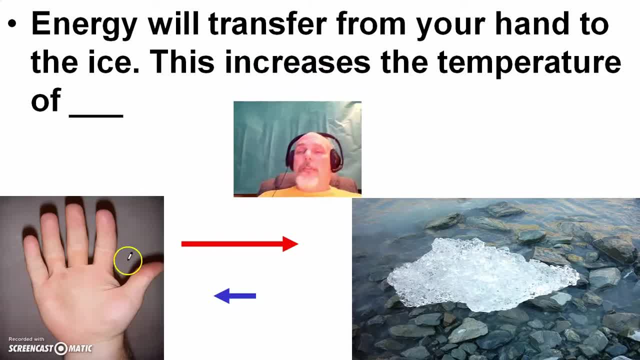 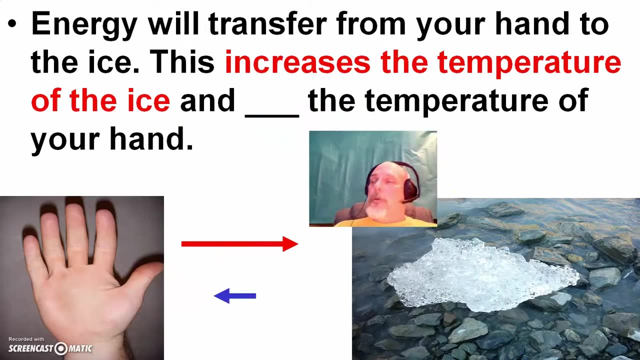 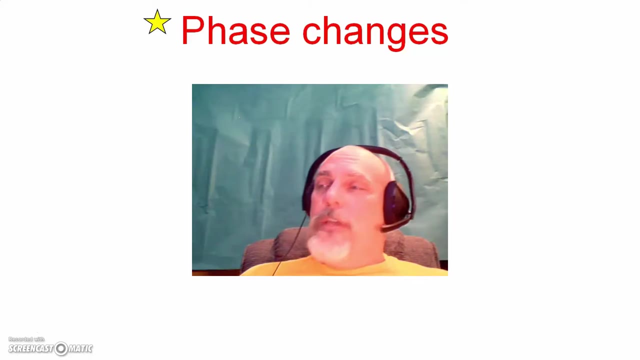 So your hand is at a higher temperature than the ice, and so thermal energy is going to pass from your hand to the ice and that is going to increase the temperature of the ice and decrease the temperature. So that allows thermal energy to completely leave the stasis over used ice. 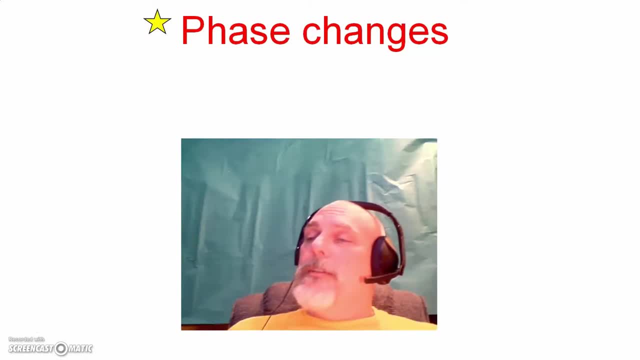 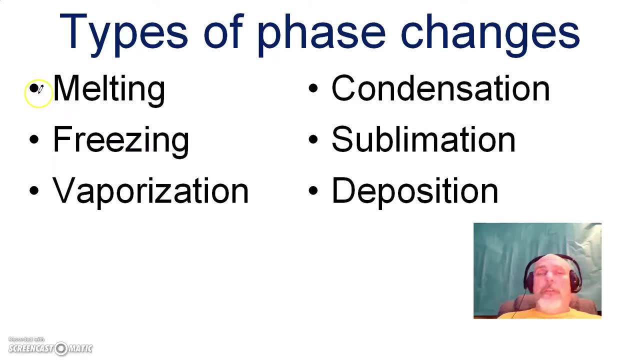 So let's look at the firstWhat you're going to be seeing is just carefully tracing what ourlya Batman stands, And what you'll see is that I've taken a look at the oneath searching, So I've gone through things that I've been able to find in clay, or I've happened to be able to figure out. 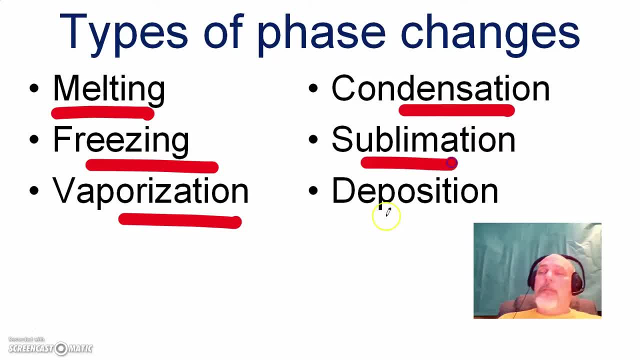 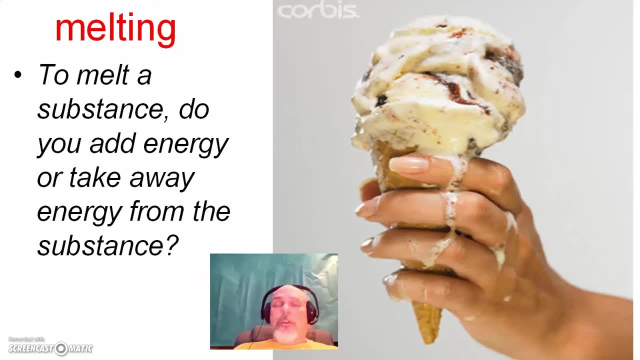 process of collecting or solving energy whenever a mass changes in water. familiar with some of these, maybe some not. today we are going to focus on melting. of course of melting is a change from a solid to a liquid. here's a question: for you, to melt a substance like this ice cream, do you add energy or 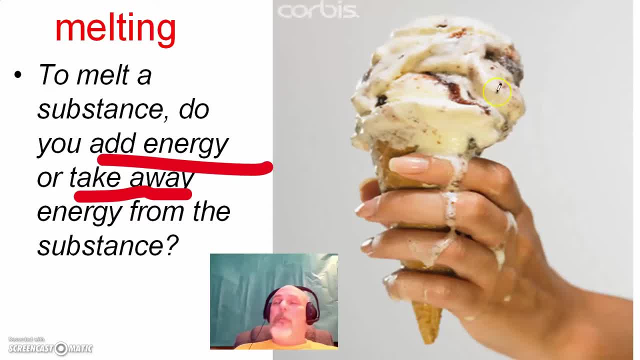 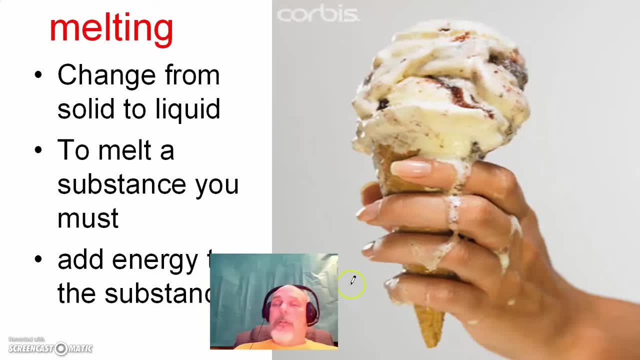 do you take away energy from the substance, or in other words, the ice cream? do you add more energy to the ice cream to get it to melt, or do you take away energy from the ice cream to get it to melt? to melt the substance, you must add energy to a substance, so we are going to increase the amount of energy. 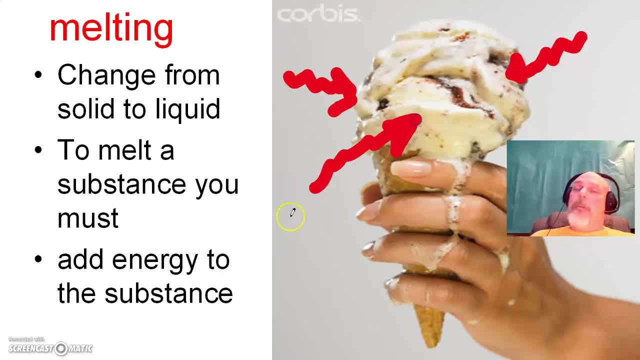 that is being added to this ice cream, and you can do that many different ways. just the warmth of the room. if it's a summer day, you're sitting out in the Sun. the Sun's radiant energy can warm up the ice cream and help it melt your hand. 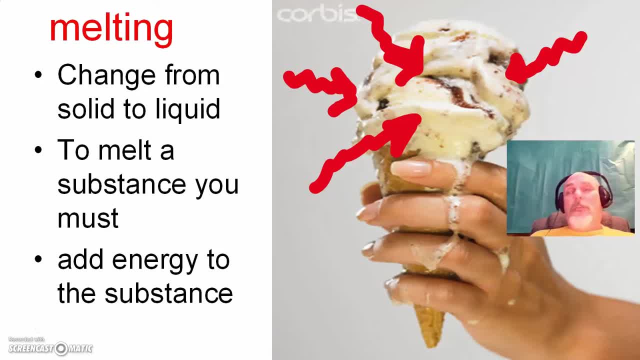 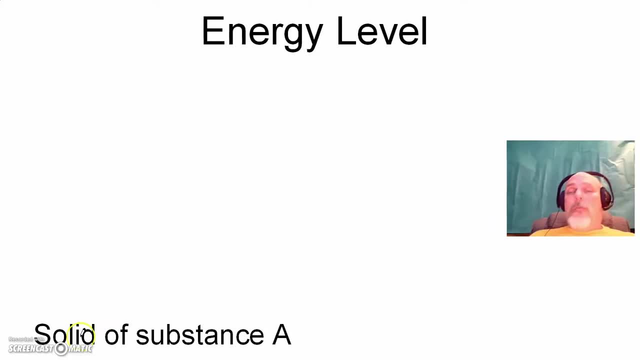 holding the ice cream. that's going to conduct thermal energy to the ice cream and allow it to melt, and this is a perfect time to talk about energy levels. so if we take away energy from the substance, we are going to increase the amount of energy that is being added to the ice cream to get it to melt. so if we 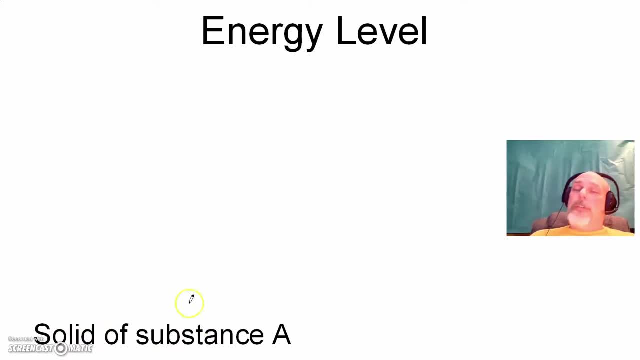 have a solid substance, let's just call it solid substance a, or in this case it could be the ice cream. the solid energy level is way down here. if we melt the substance and it becomes a liquid, the liquid of substance a is at a higher energy level than the same solid, in this case the ice cream. if it was liquid ice. 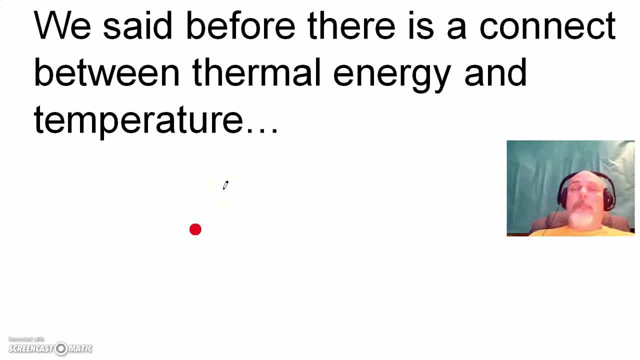 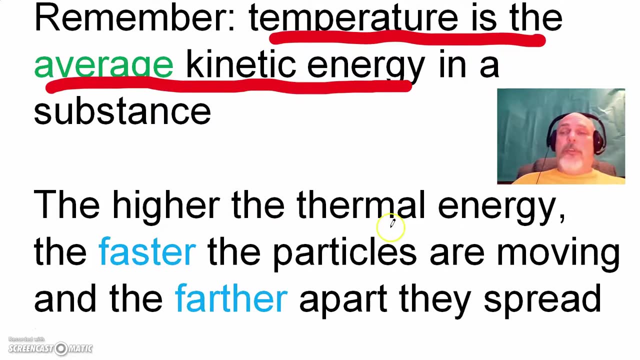 cream is going to be at a higher energy level than the solid ice cream and we are going to want to herbalcend it and we're going to want to mix it with ice cream and the solid ice cream are going to draw that volume up to about. 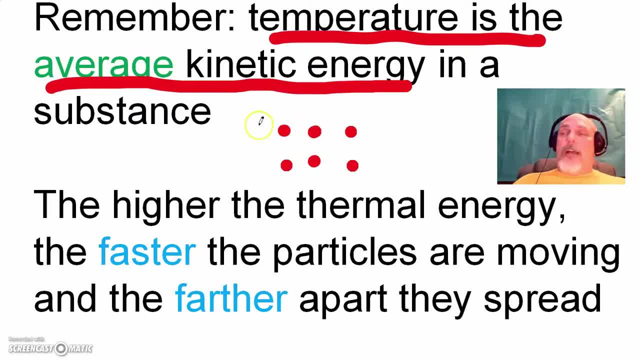 zero. it can be either one, water or other components. you will have two in the particular. Set it in both of these dropdown boxes and you'll be watching the cycle. amazing number and how we are going to increase the temperature between the thermal energy and the temperature of a substance. quick review: temperature is. 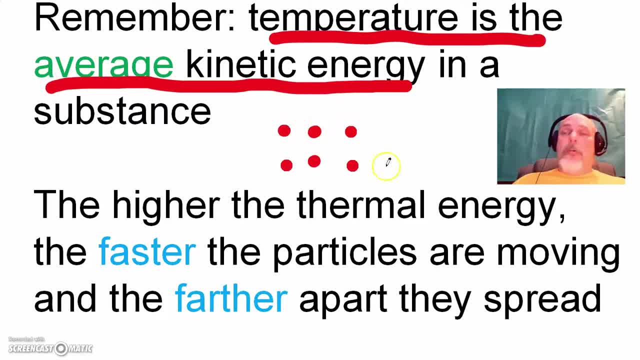 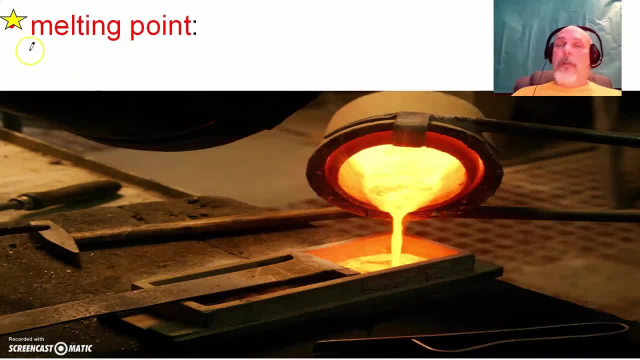 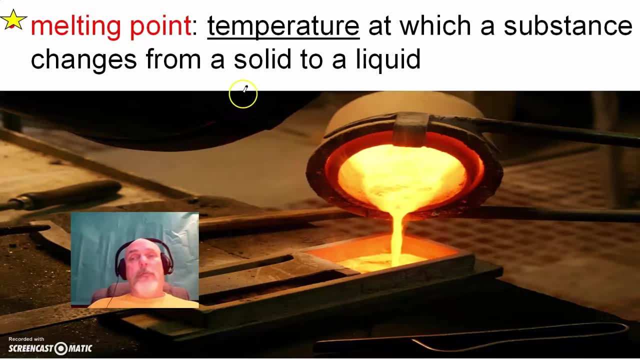 they're gonna vibrate more and they can get a little bit further apart from one another. they can spread out. which brings us to our next vocab term is melting point. the melting point is the temperature at which a substance changes from a solid to a liquid. this is a temperature. it's gonna be a number, the 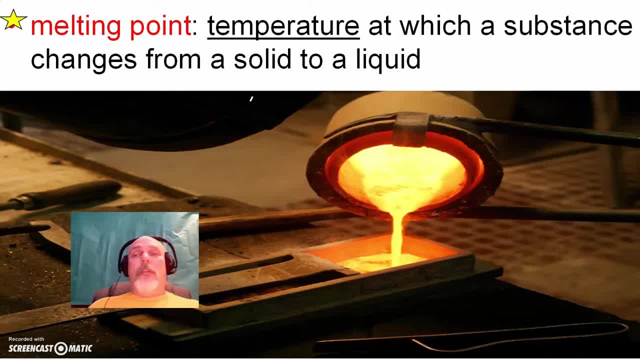 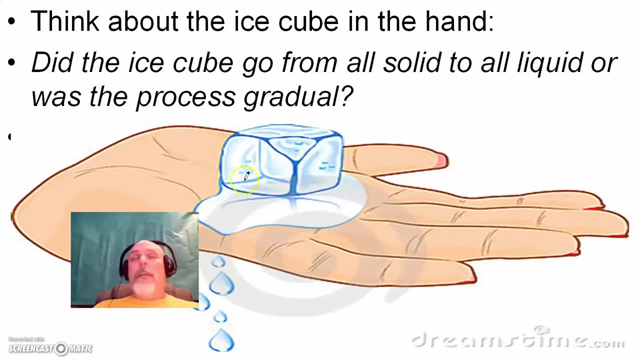 melting point is going to be a number of some sort, and this is going to be when that solid actually gets enough vibration, enough motion, enough energy to actually break free from the attraction to its neighbors and become a liquid so it can actually change position. and if we go back to think about our sit right, 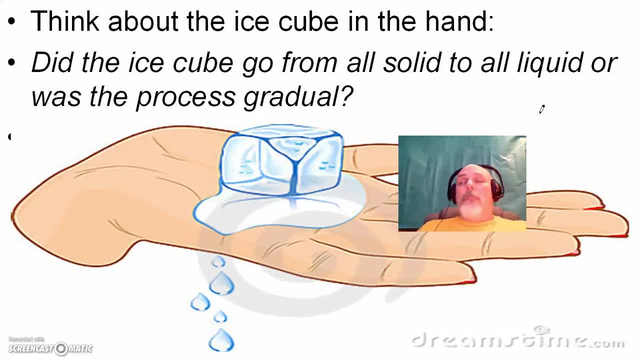 here. if I go back to think about our ice cube in the hand. did the ice cube go from all solid to all liquid, or was the process gradual? just look at this picture right now. you can see that there is some particles of water in liquid form and there are some particles of water in 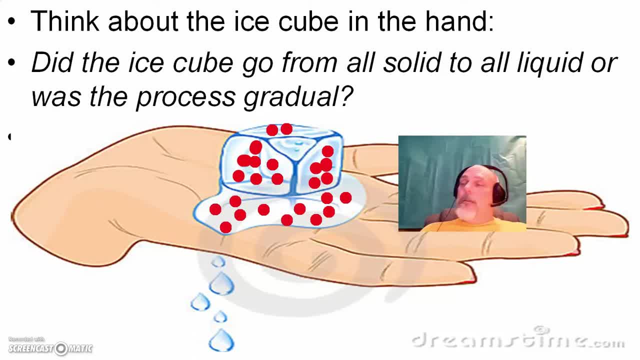 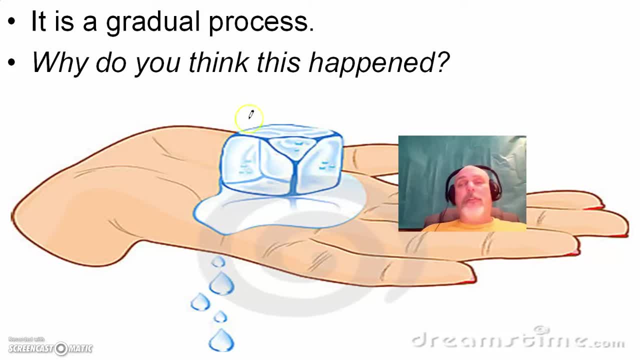 solid form and we could see that, so that we could see that as a gradual process. why is this a gradual process? why doesn't it just happen instantly where the ice becomes a big puddle of water, or this becomes softer, or anything like that? let's think about that. well, here you have all these particles in here. 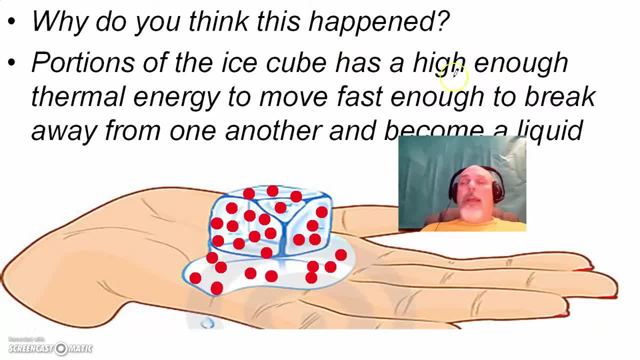 and portions of the ice cube may have a high enough thermal energy to move fast enough to break away from one another and to become a liquid. so these particles down here that are actually in contact with the hand, these are probably going to be vibrating a little bit faster than the particles here. the 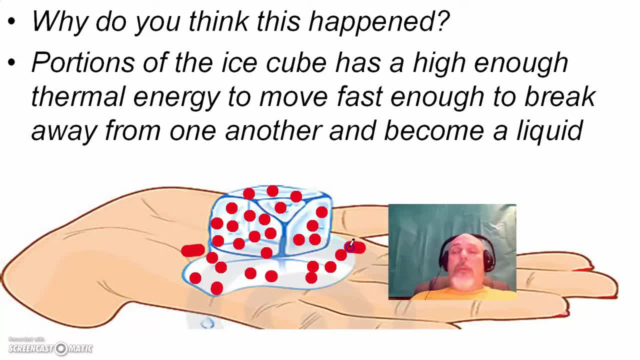 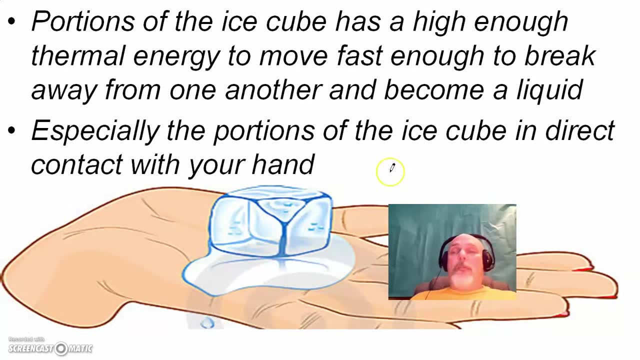 reason why is that they are in direct contact with the hand, so they're going to be getting thermal energy conducted directly to them. the vibrating particles in the hand are going to vibrate and increase the thermal energy or the motion of those particles, and those particles get fast enough that they 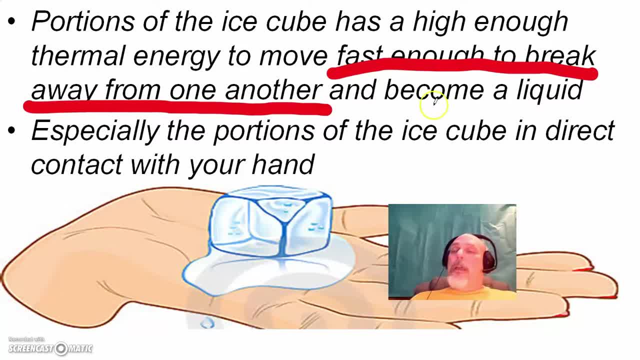 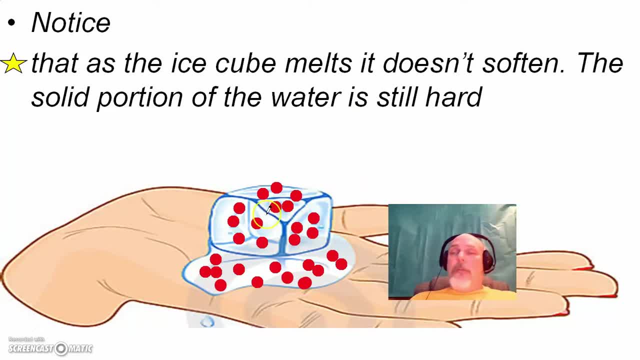 can actually break away from one another and become a liquid. an important thing to notice is that as the ice cube melts, the ice cube does not soften. the solid portion of the water is still hard. so this solid, the ice cube is still hard. it's not softer than the ice cube was before. 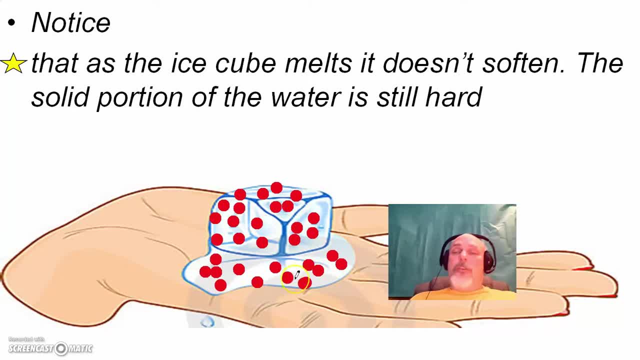 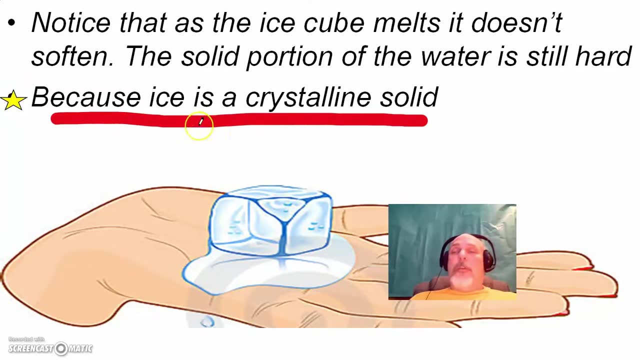 the liquid particles can change shape and move around, changed position. they are not in the same rigid, fixed position as they were in the solid. the ice cube does not soften as it melts because it is a crystalline solid. the particles will stay in a repeating pattern and stay. 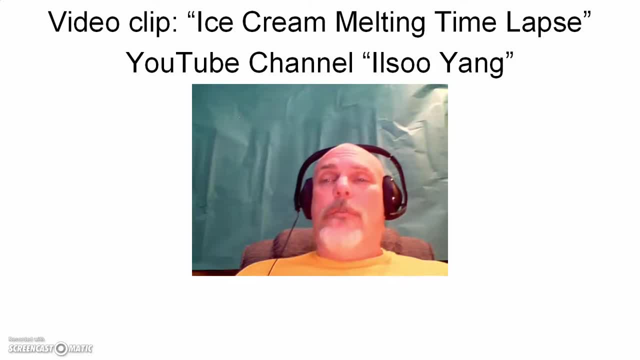 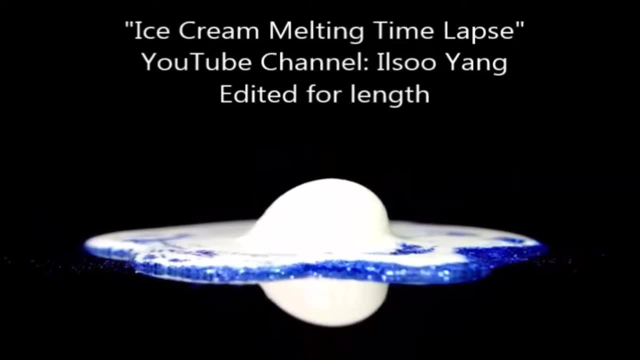 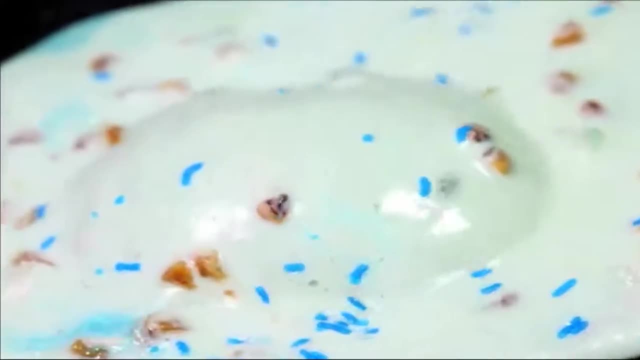 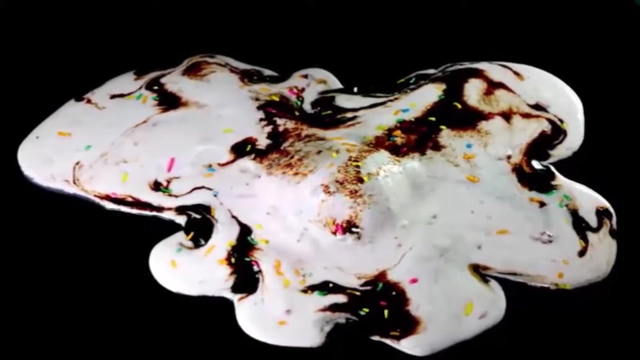 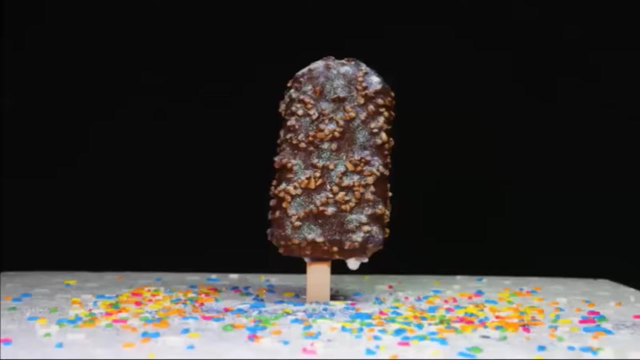 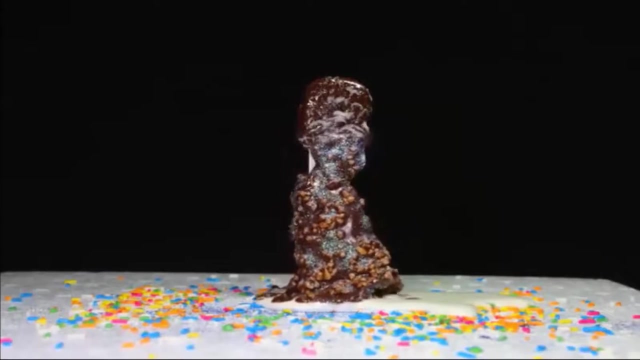 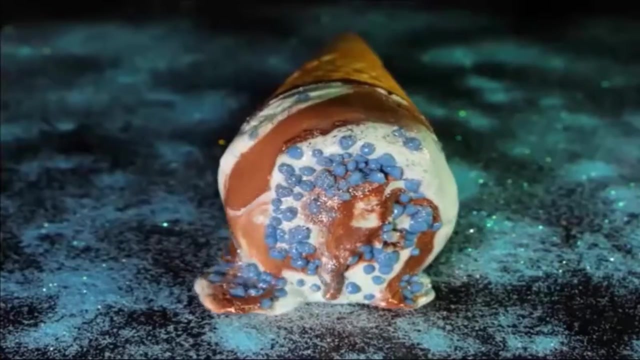 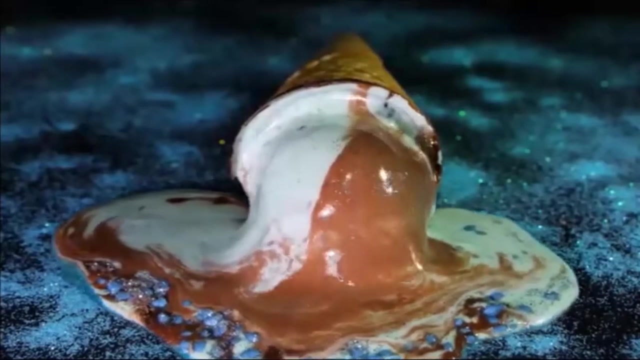 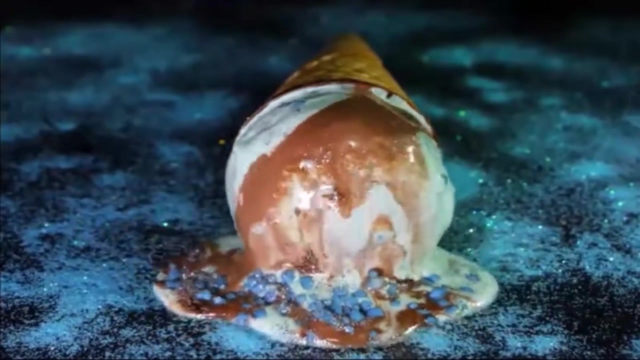 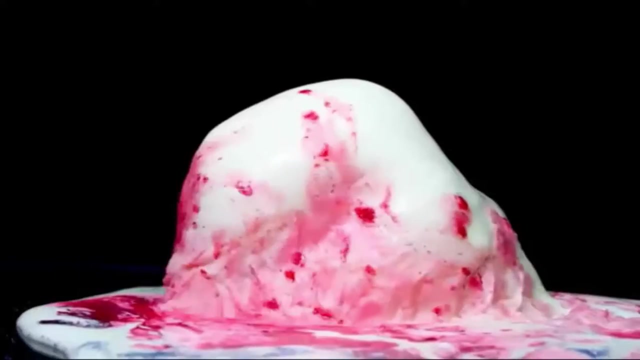 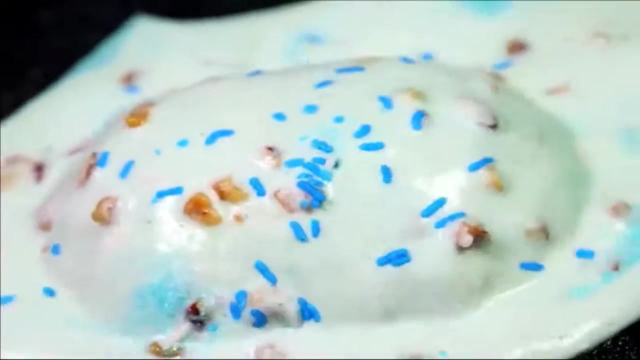 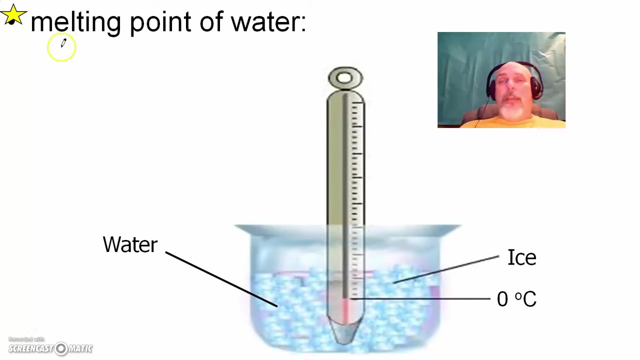 that position: Crystal and solid. Let's take a look at this video: Ice cream melting time lapse. Ice cream melting time lapse- Melting point of water. Now, we should remember that melting point is an actual temperature, So melting point of water is going to be the temperature at which water goes from a solid. 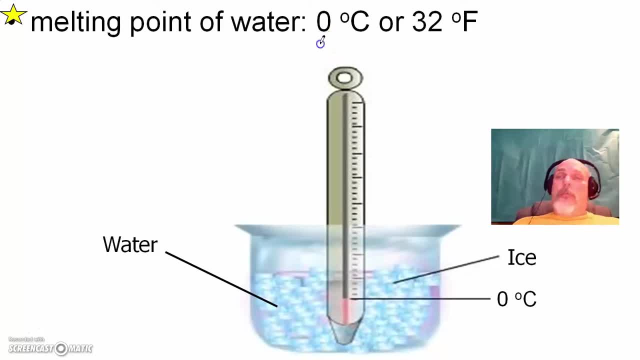 temperature to a solid temperature. So melting point of water is going to be the temperature to a liquid. These numbers I would expect you to remember. So 0 degrees Celsius or 32 degrees Fahrenheit, They are both exactly the same temperature, It's just a different measurement. 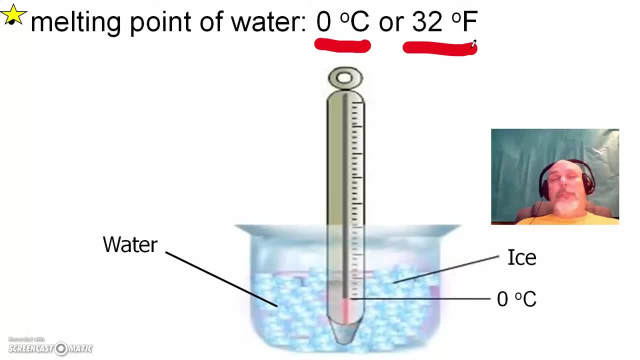 scale, Kind of like: if you have 2.54 centimeters is equal to one inch. Please note that at zero degrees- that's the temperature the thermometer is at in this drawing- that there is solid ice and there's also ice in liquid form. You are going to have both liquid water and solid. 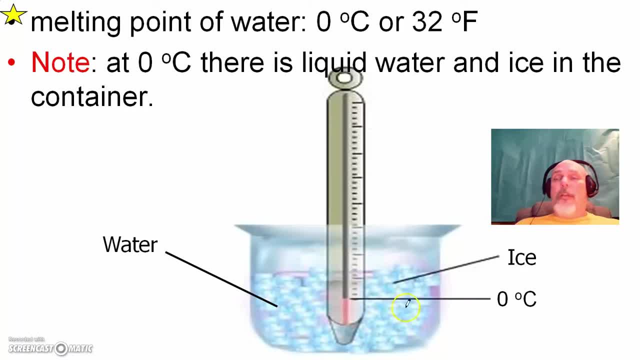 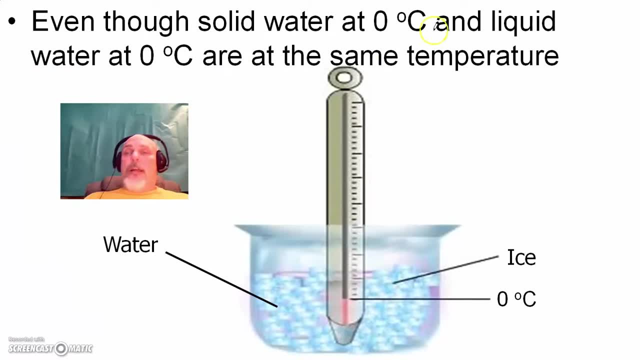 water or ice in a container at zero degrees Celsius. Water may be a liquid or a solid at zero degrees Celsius. Even though solid water at zero degrees Celsius, liquid water at zero degrees Celsius, they're the same temperature. Are they the same energy level? Well, no, they are not. 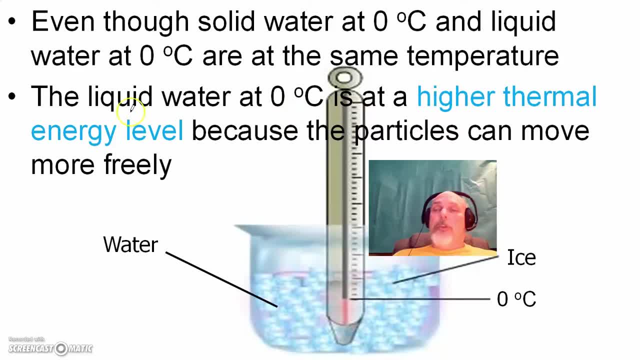 The liquid water is at a higher thermal energy. Liquid water at zero degrees Celsius is a higher thermal energy level because those particles can move. The particles in the liquid are able to move around and change position, whereas the particles in the solid are still locked into that rigid crystalline structure. They are not able to. 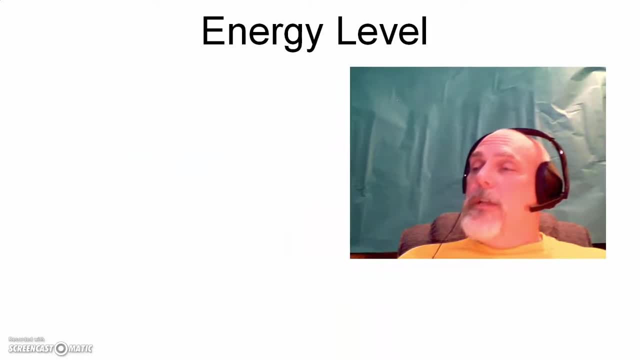 move freely And let's go back to our little handy dandy energy level chart And you can see that the solid of substance A. now we can substitute ice, So the solid ice is going to be at a lower temperature. The solid ice is going to be more cold than yours. The cold ice will be at a lower temperature. 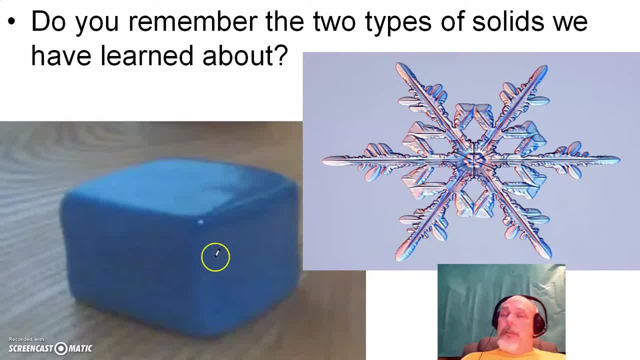 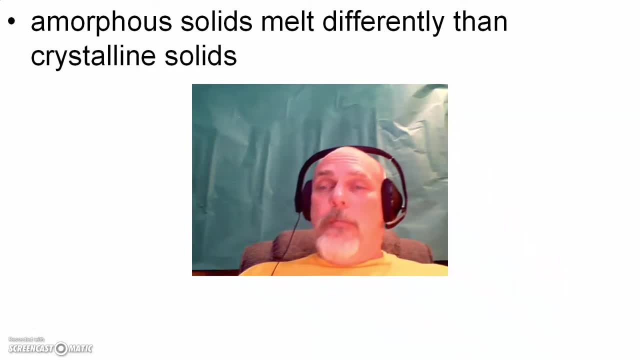 And the cold ice will melt. And just to give you guys an idea of what solid ice is: solid ice is a solid ice that is not in water, It's not in ice. It's a solid ice that's going to melt when it melts, because when they melt it will melt. So in the solid ice we get, 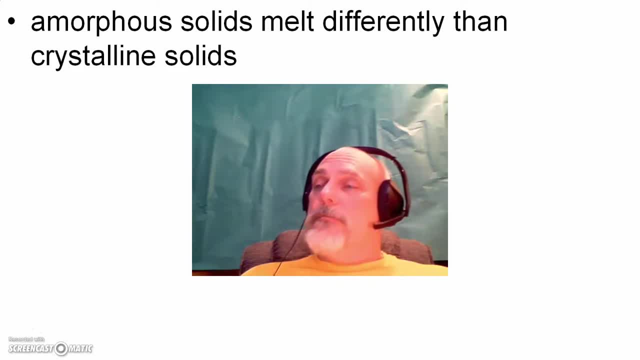 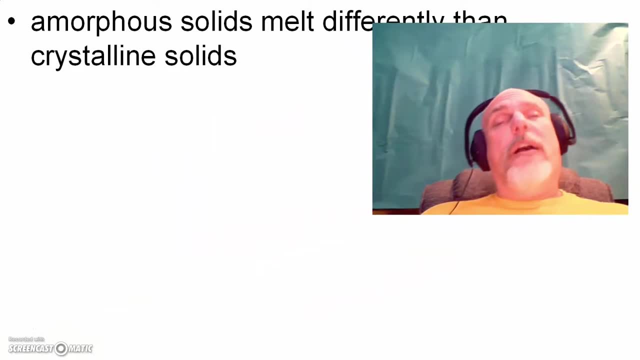 a little bit of water, as well as a little bit of ice that melts. In the solid ice there is a little bit of ice that melts, And this one. we get a little bit of ice that melts, which is called as solid ice. The solid ice does not melt. when it melts, We keep doing. 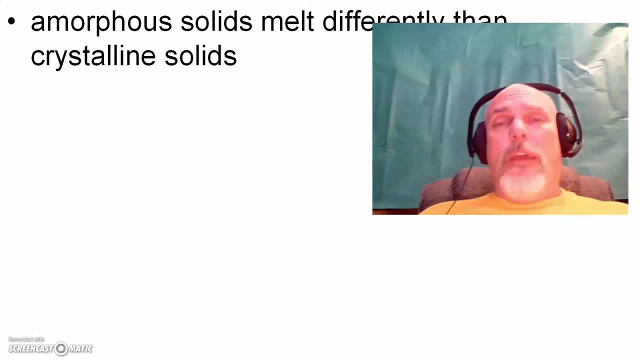 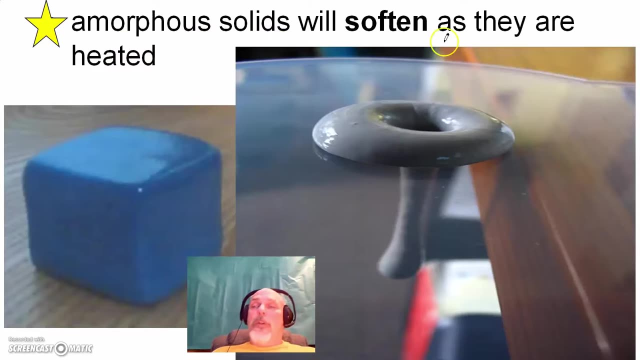 or plastic. as you heat up or warm that rubber or plastic or wax, candle wax, clay, the clay candle wax will start getting softer, even before it becomes a liquid. you can kind of see some pictures of that right here. amorphous solids will soften as they are heated. 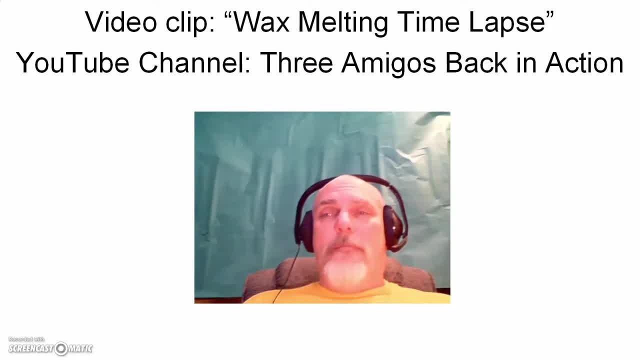 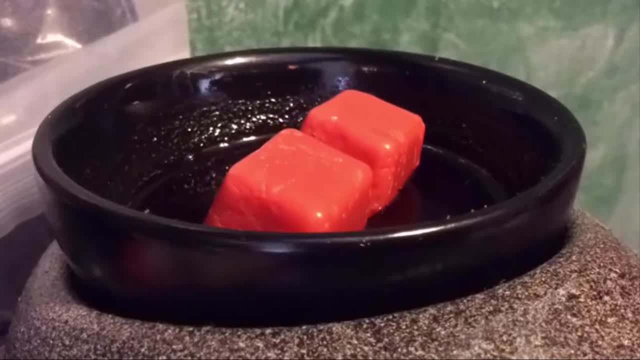 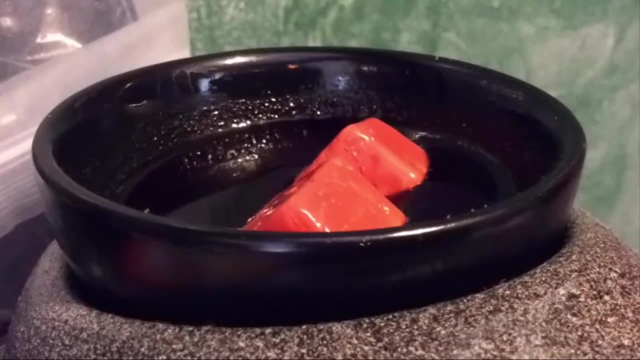 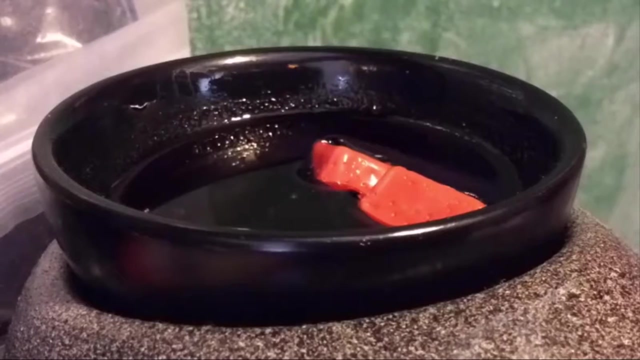 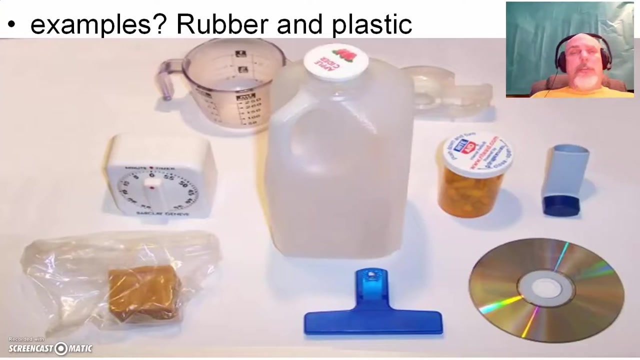 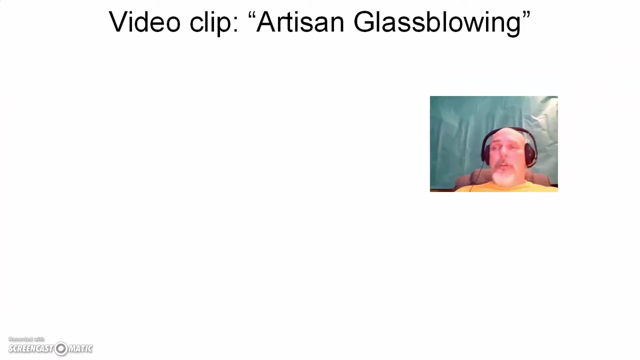 here's a video clip: wax melting time lapse- lapse, lapse lapse. example. examples: bandaging banned for less than a week. examples. examples of amorphous solids: sleeping habits, solids, rubber, plastic glass. glass is a good example. got a cool video clip for you to check out about artesian glass blowing. 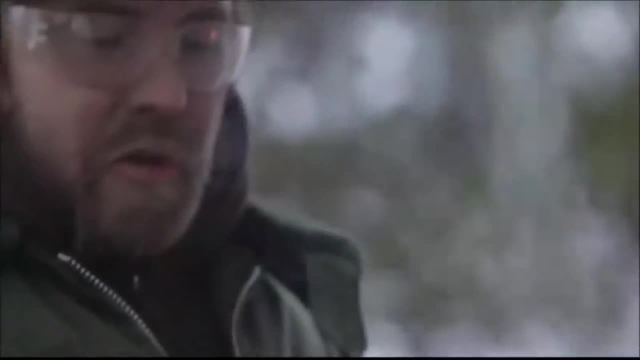 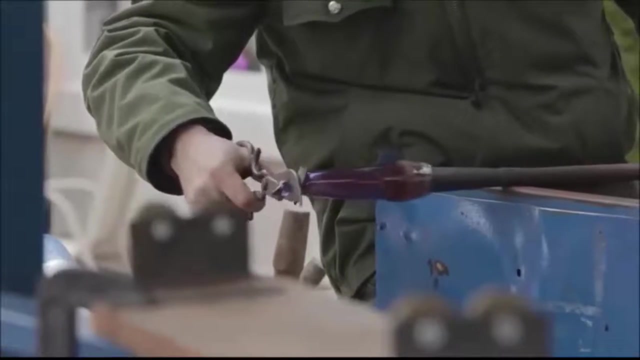 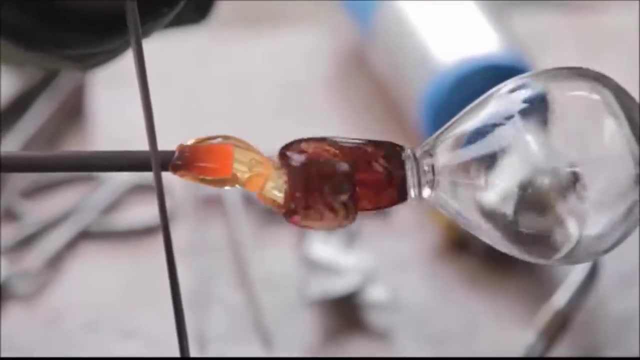 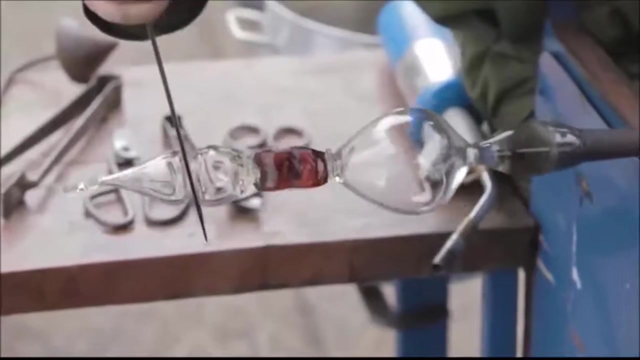 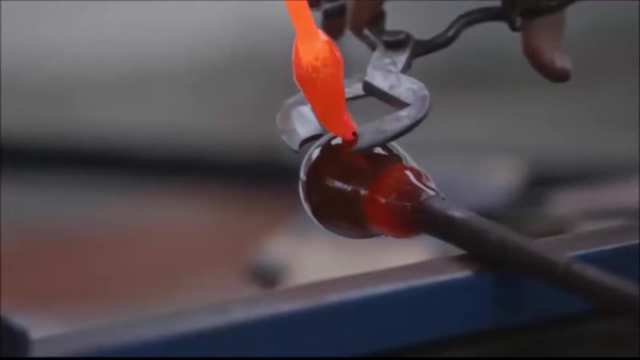 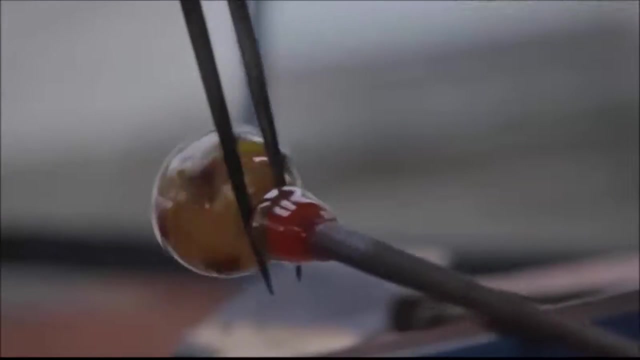 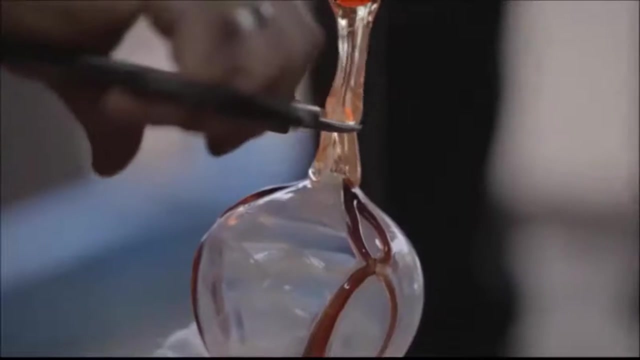 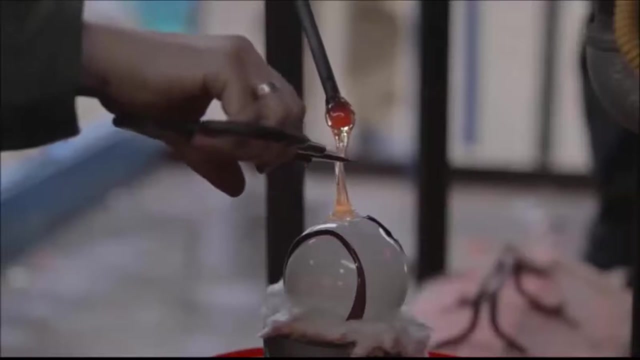 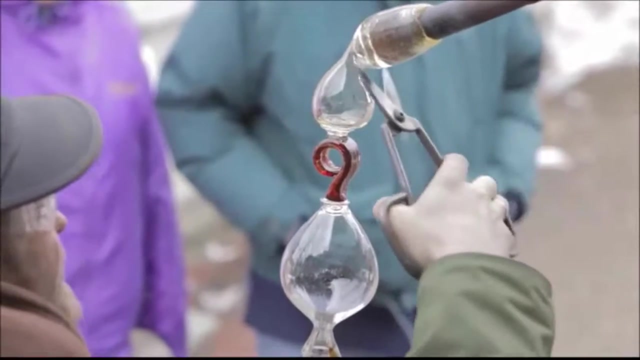 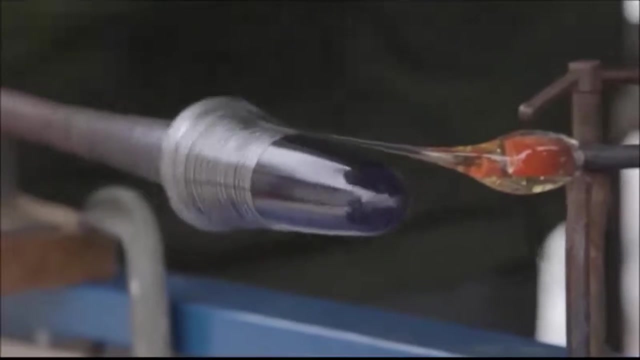 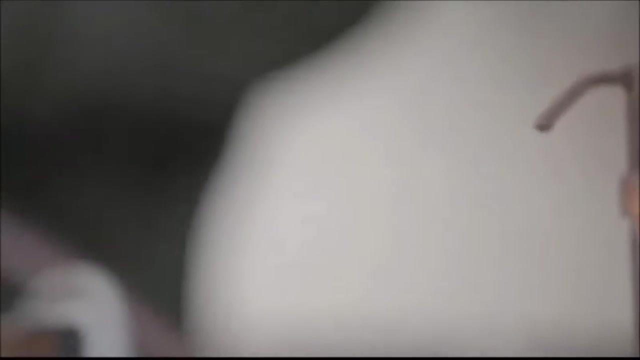 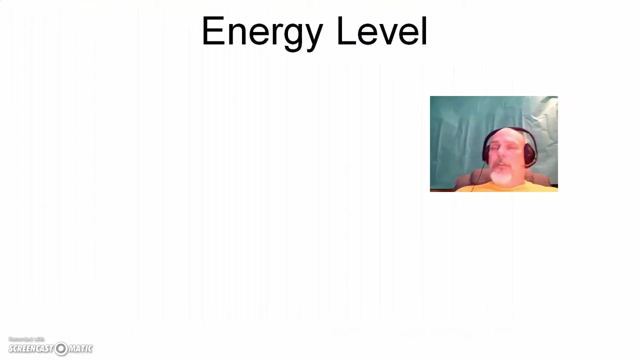 you. you, moving back to our energy level chart, solid of substance, a, let's say this is a glass in this case. so so solid glass is at a lower energy level, then liquid glass. when you melt the glass, it is at a higher energy level because the particles are able to. 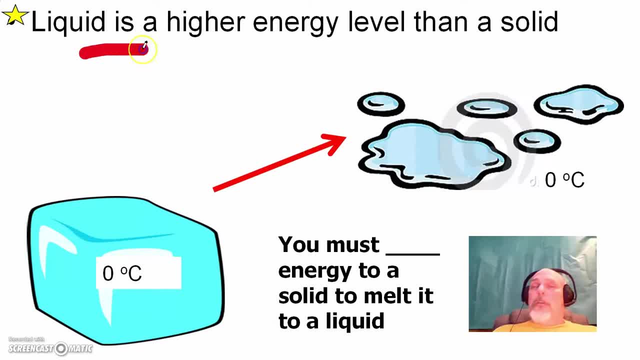 move more freely and change position. liquid is at a higher energy level than a solid. you definitely need to know that. here is a block of ice. if you remember, the freezing point or the melting point of a block of ice is zero degrees celsius, zero degrees celsius. piece of